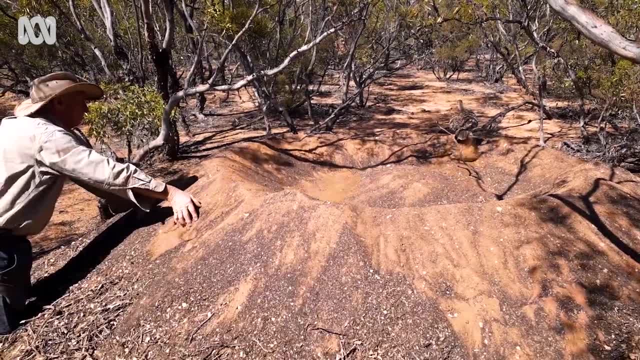 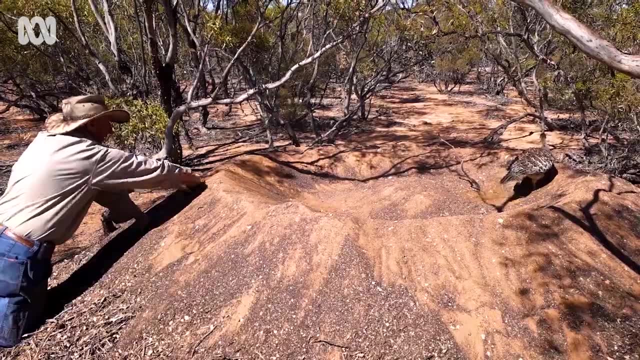 I could help him fill in his nest in the middle of summer when it was stinking hot and he had to get it filled in. He was absolutely exhausted, still trying to fill it in, and he let me help him. How hard is it to find a mate when they're out here in such remote country? 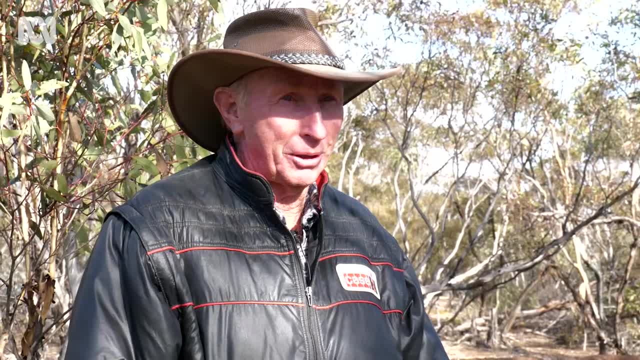 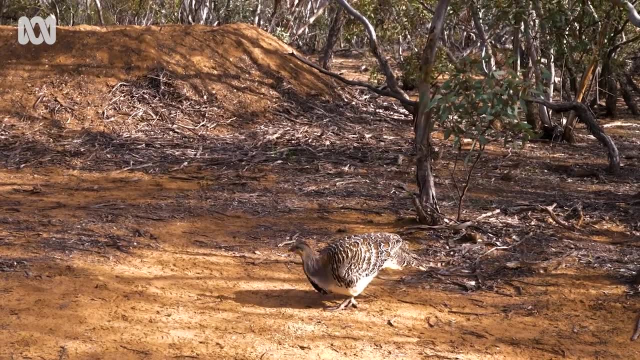 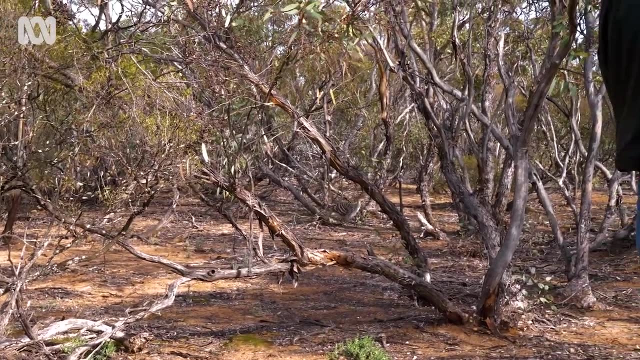 She didn't mourn too long. She must have just got onto the internet and got onto: Mally Fowl Wants a Husband, Yeah, or something like that anyway, and she had one within a fortnight. He's crashed up. He's still pretty suspicious. 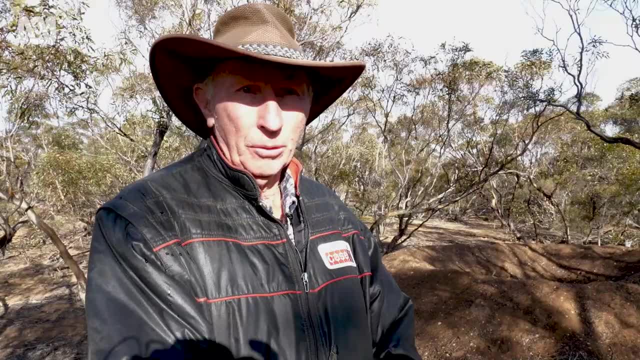 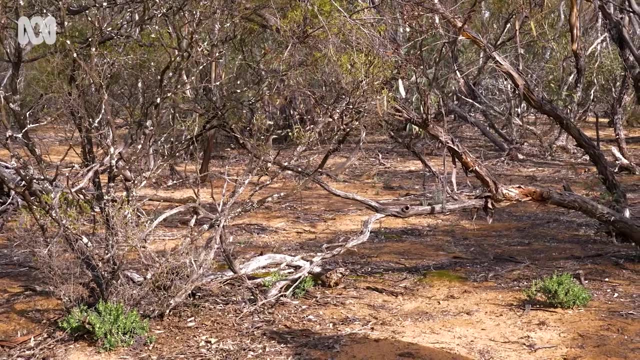 The thing with their colour and their patterning makes them perfectly camouflaged to hide in this sort of area, doesn't it? Oh, absolutely, I could say to you: there, it is there, and you can't see it until such time as it shifts. 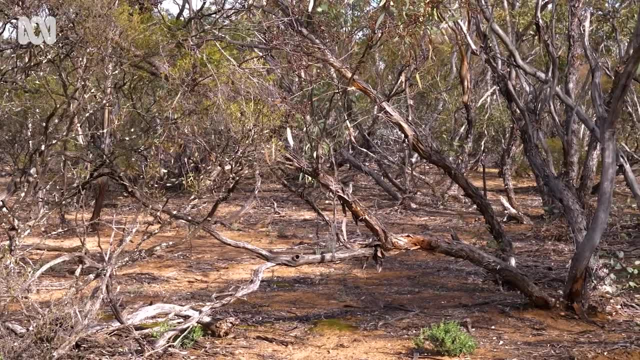 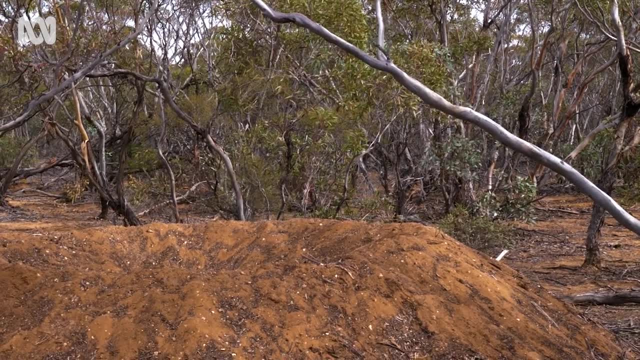 You know they're absolutely perfect and they're experts at standing dead. still, Do you think this is a bit of a haven for the mallee fowl compared to other areas that they're really under threat? Well, I don't know. There used to be a lot in the big desert. 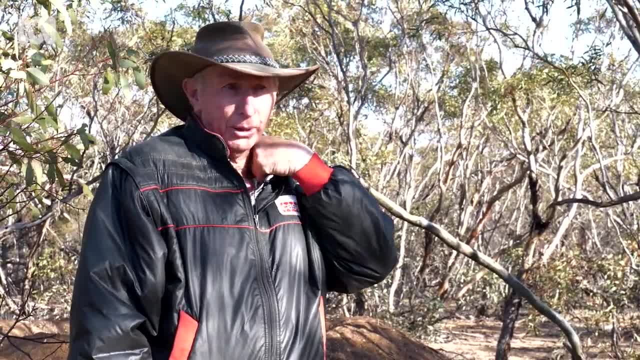 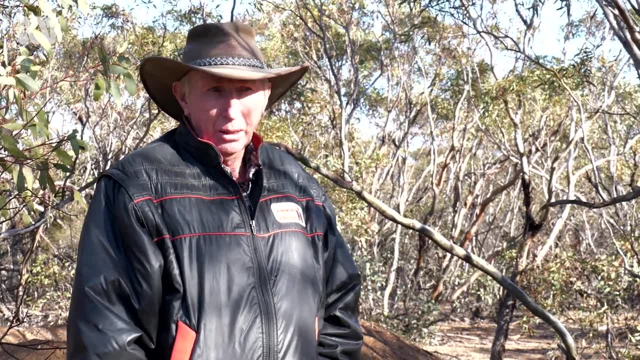 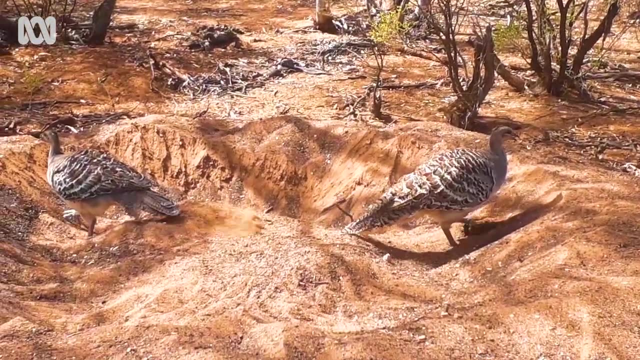 We used to know where they were in the big desert, But then, when the fires were there in 2003,, the birds were all flying over us and heading this way, and then suddenly a lot more nests appeared up here. So I don't think that they've gone back to the big desert yet. 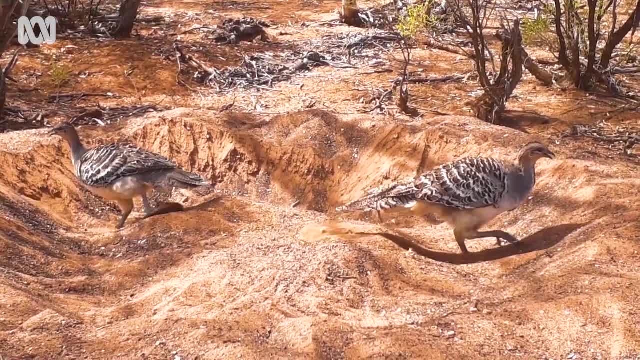 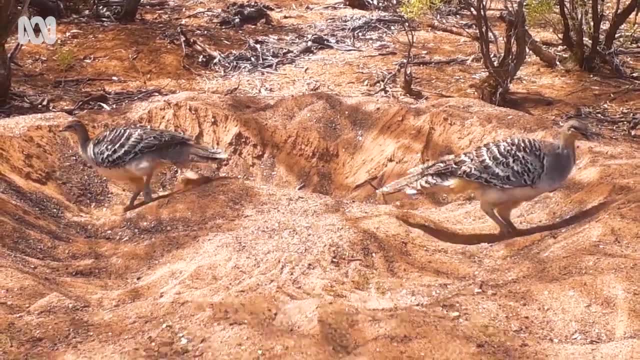 How far away is that? They would have travelled quite a distance. Yeah, probably 30 kilometres. So mallee fowl can fly. Yeah, and the interesting thing about a mallee hen: it can fly like a helicopter straight up, like that. 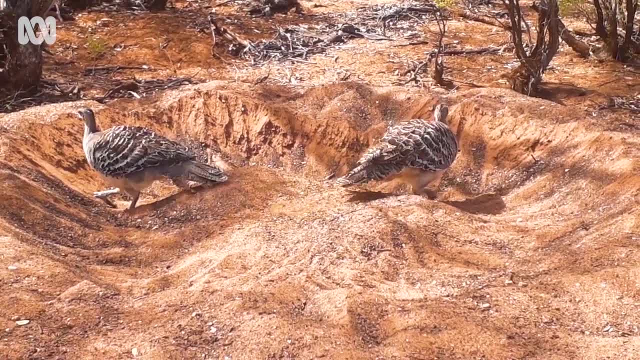 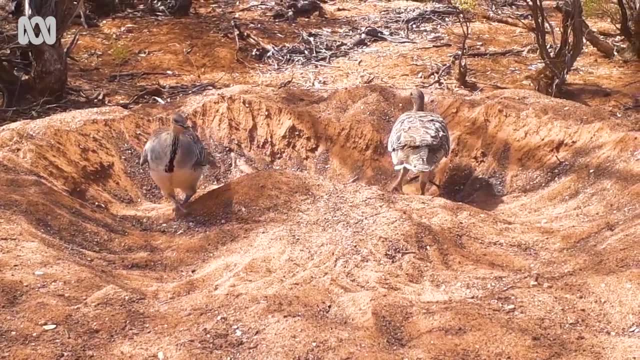 It roosts in the trees at night time, so the foxes don't get them, Um, But normally they won't fly, unless you really frighten them. They'll just run off into the bush, And then they're so good at camouflage, they just stand there. 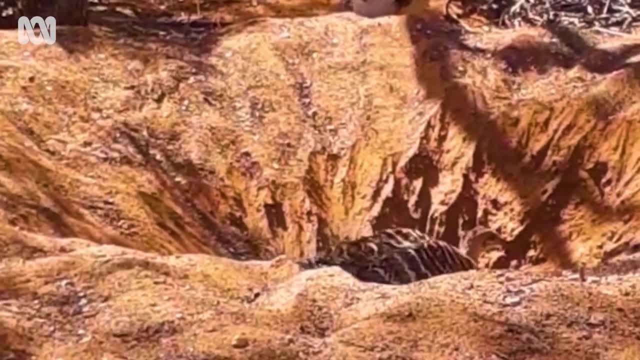 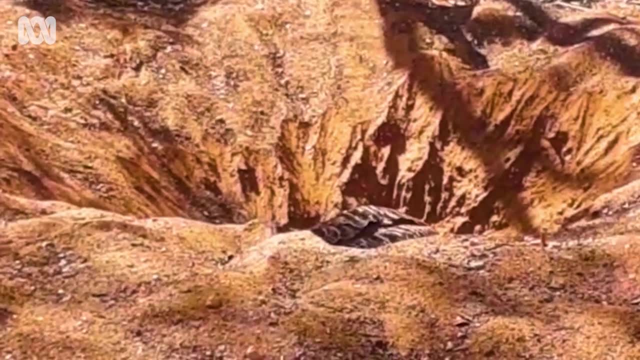 and you don't see them anymore. We're looking at a female mallee hen just laying her egg. now You'll notice she pushes the wings of that right out against the side of the wall. The poor bird. when she's laying egg it's like giving birth to an elephant. 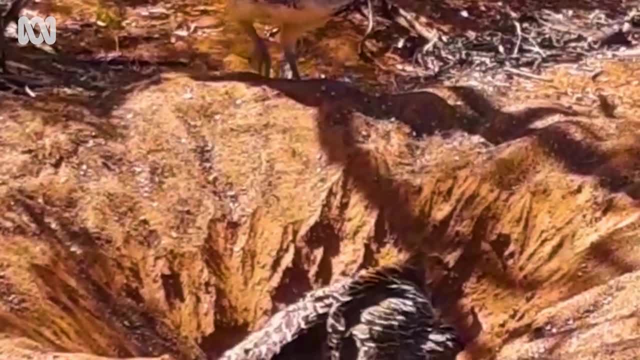 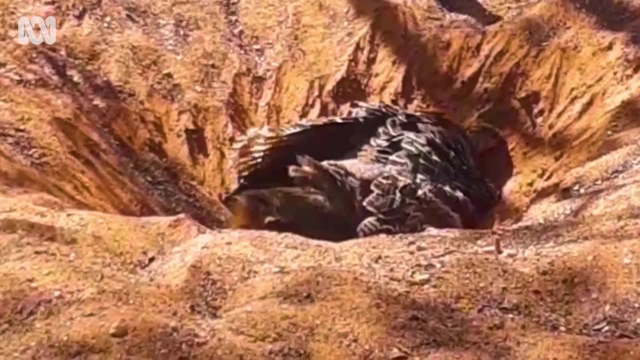 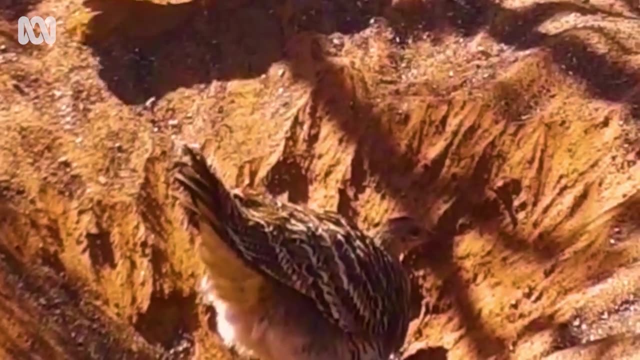 And then she's exhausted By the time she lays eggs. she can hardly get out the nest, Poor thing. Oh well, the dedication of a mother That's a male up the top waiting for it to fill the nest in as soon as she's laid it. 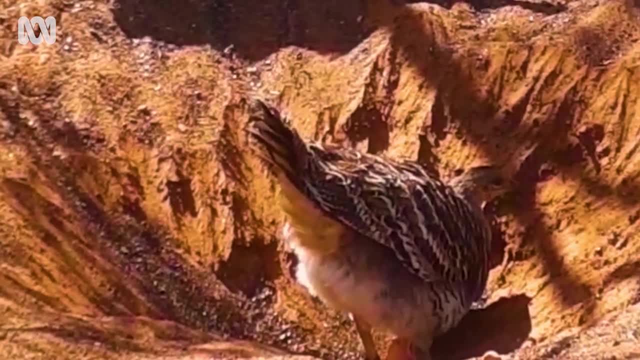 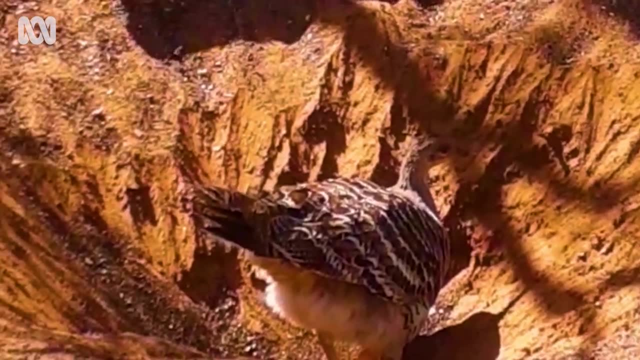 I estimate they shift a tonne of sand a day for 11 months of the year and they knock off Because they have to open this nest to test the temperature. How many eggs do they lay after all this work? 20 or 30.. 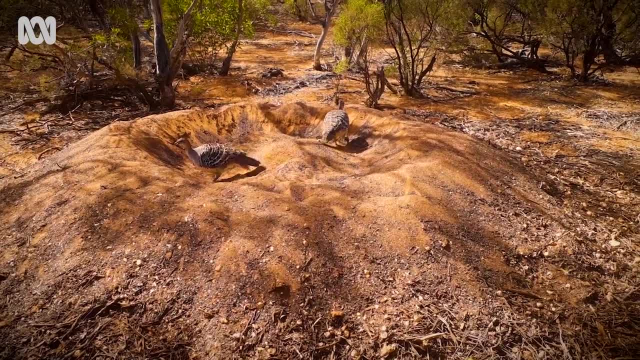 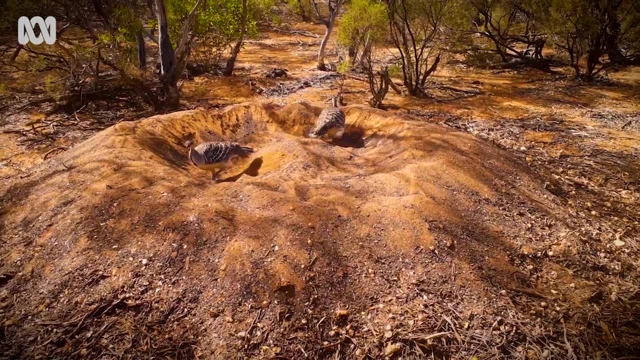 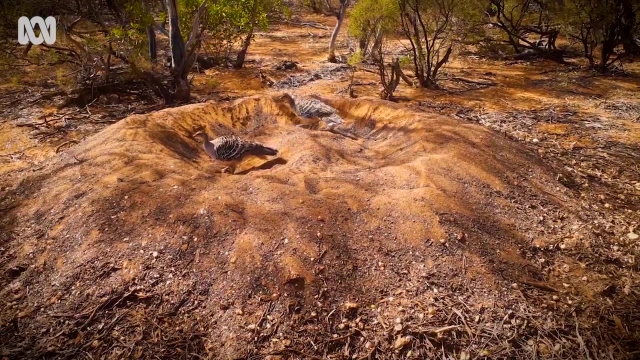 One every three or four days. They lay and then they take 50 days to hatch. The nests just get bigger and bigger because they keep raking mulch in and that breaks down and makes them more soil And they just keep building the nest up higher and higher. 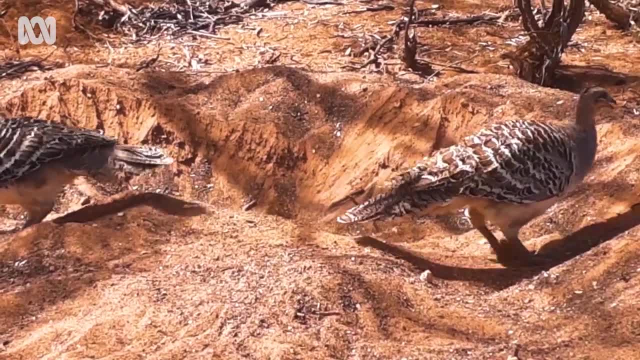 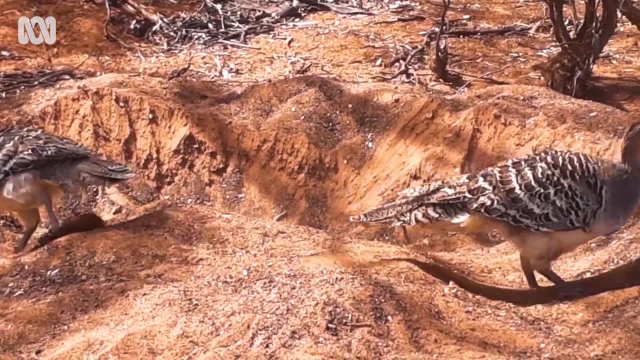 Is it the breaking down of the compost that keeps the nest warm? Yeah, it's the warmth of the material breaking down that hatches the eggs. The nests don't sit on the eggs at all, But out here in the desert it gets pretty hot, so that's why they dig it out. 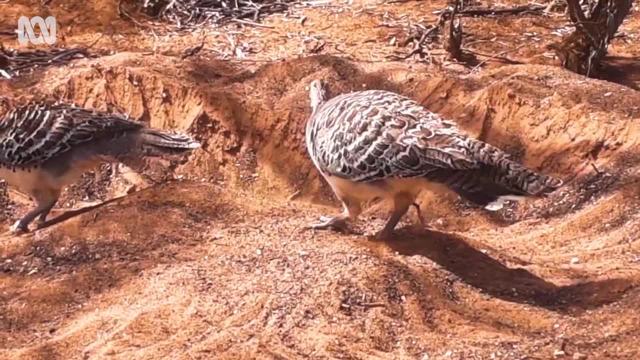 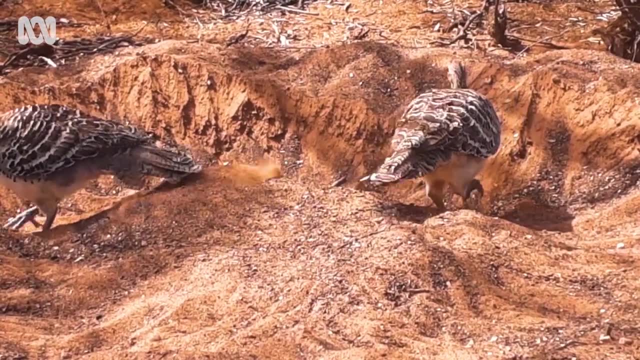 I know. if it's going to get too hot, they put sand on so that the heat can't get in there. If it's too cold, they scratch it off in the morning and then scratch it back in before evening, before the sand starts getting cool. 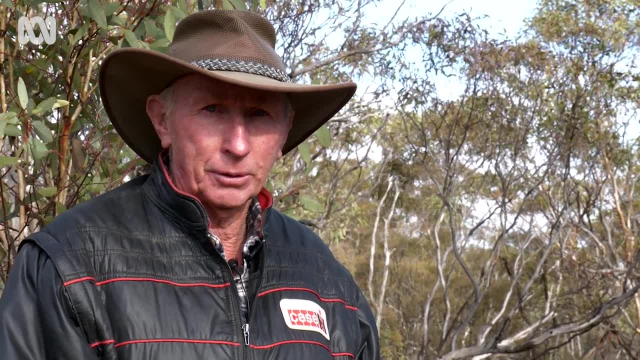 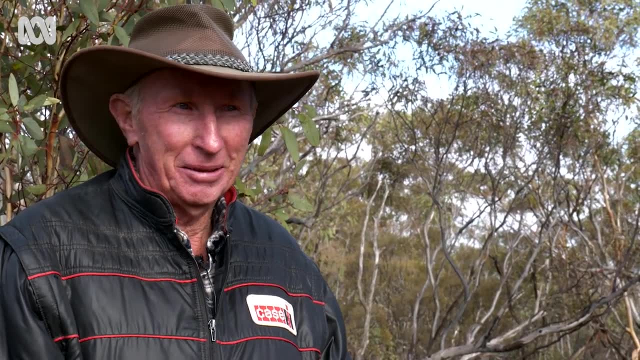 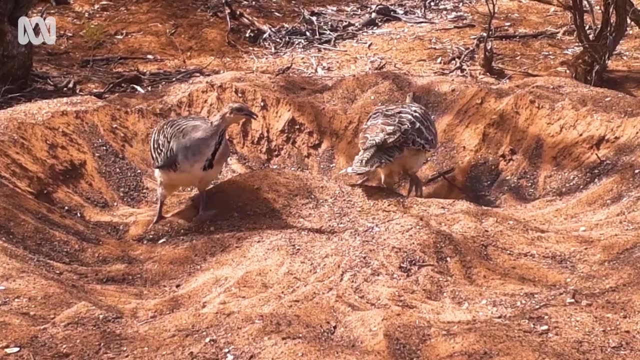 So that's how they regulate the temperature. So it's like geothermal incubation. I would dare say you could say that They're pretty intelligent birds then, aren't they? It just blows you away that they know how to do all this from birth. 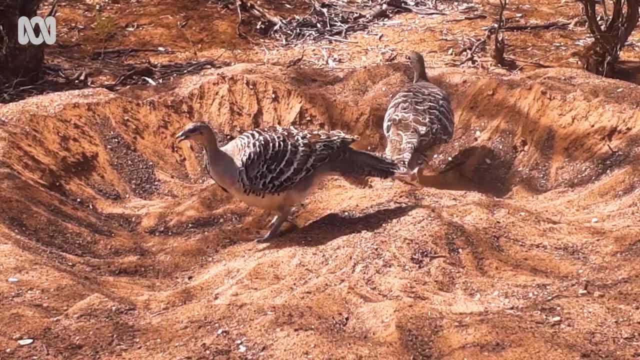 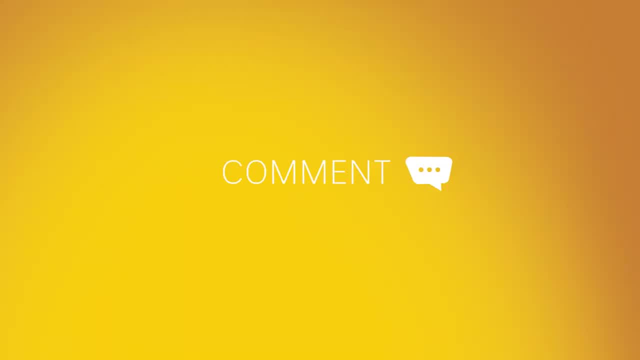 The young can fly within about an hour of hatching. It's really putting us humans a little bit to shame, isn't it? Yeah, I mean, the world's not made of this stuff. I mean, if it's going to get cold, then it's still going to be hot. You're right. The temperature's going to keep getting colder and colder And when it gets colder it's going to be difficult to get the nests to come up. They're going to get all wet. When they get up, they're going to get all wet. And they're going to get all wet And they're going to get all wet. So you could say that's how they get the nests to come up. But I would dare say that when they get cold they start getting a little bit more wet. Yeah.